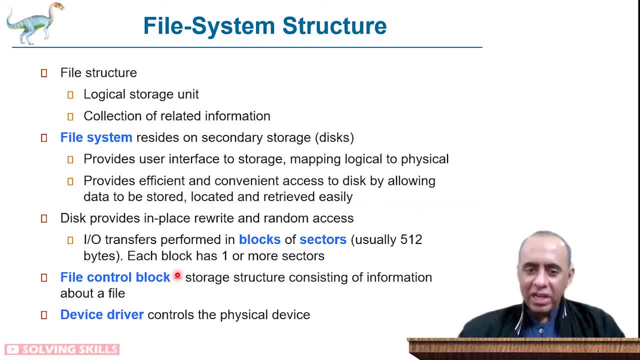 the file control block for every single file inside your disk, so every file will have what a file control block, just like we said that every process has a process control block and anything that happens below that level. how the logical blocks are maintained, how they're accessed, how they're mapped from logical address to physical address. 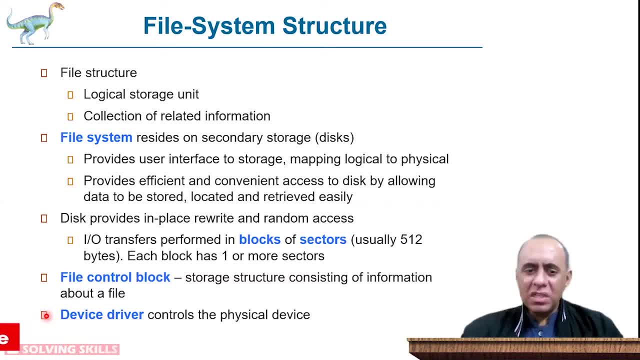 we do not worry about that. we don't need to worry about that, because there is a tiny computer inside that physical device which takes care of all of these things, and there is a supporting software also installed, installed in your operating system, which is called the device drivers, which takes care of all the underlying hardware issues of the physical disk. so we're not. 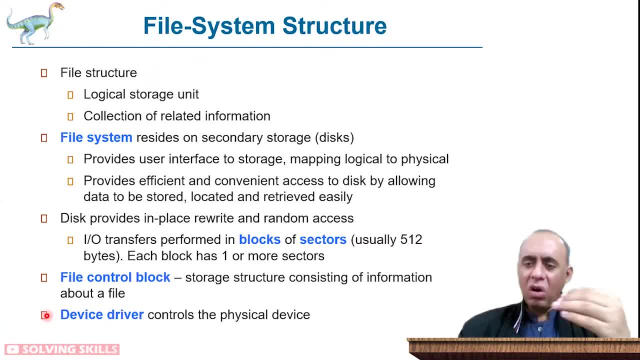 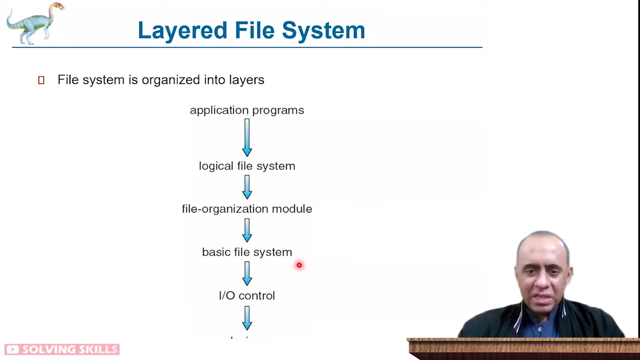 concerned about that. we simply say that we can see the existence of the physical drive using this device driver as a, as a software entity, and we are simply sending request of read write to that software entity as logical blocks. right, and this is again a representation and of how what i've just said can be represented, that this part, the i o control and 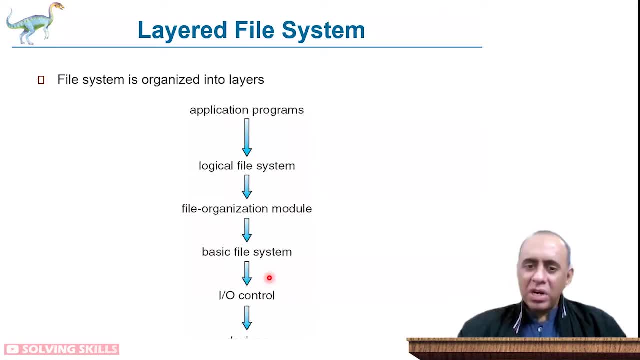 device part is we? we don't bother about that, but we are actually on on on this level, actually inside the logical file system as well. so these things will be inside the file system: how the file organization module is implemented, what is the basic file system. so we will be looking at the 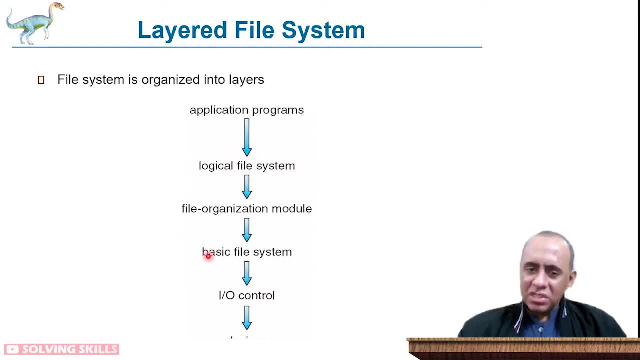 logical file system and these informations we- although we are going to study in this chapter how these are implemented- but the users? they only see the logical view of the files which, in the case of a graphical user interface, you see as an icon or, in the case of the command line, 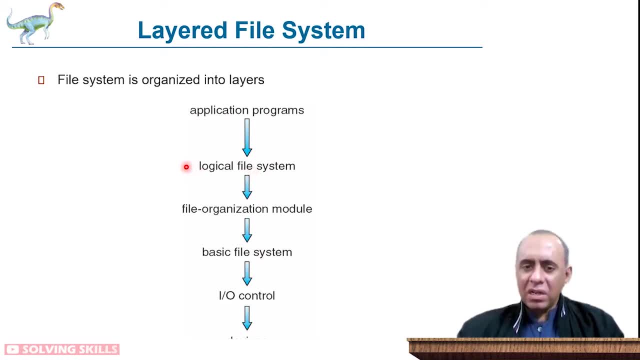 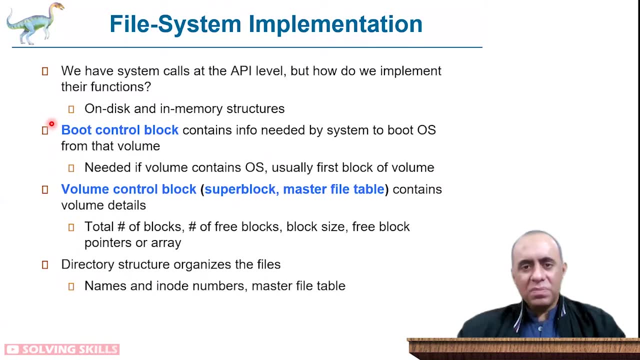 interface you see as a file name. so this is the, this is that part. but these parts we will be seeing in this chapter. so let's see what those are. so first there is a boot control block, so we have system calls at the api level. but how do we implement their functions on disk? and 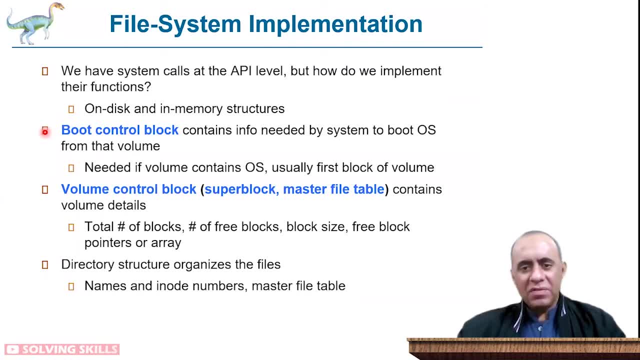 memory structures. we have a boot control block which contains information needed by system to boot the operating system from that volume. and this is a system that is used in the operating system, that volume. it is needed if volume contains operating system. usually first block of volume and then there is a volume control block which is the super block or master file table contains the 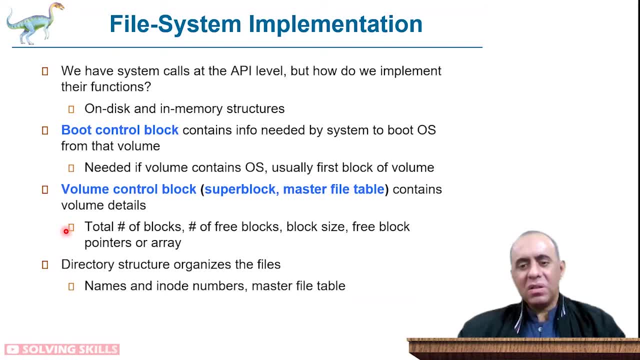 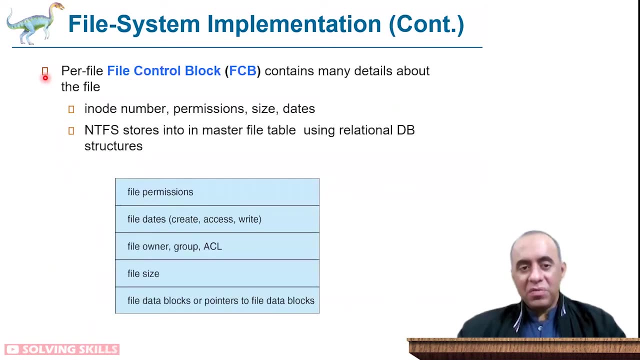 volume details like the total number of blocks, number of v blocks, all the information about that. that disk and the directory structure organizes the files using names and their ids, called inode numbers and master file tables. and this is a how a file control block or an fcb look like it. 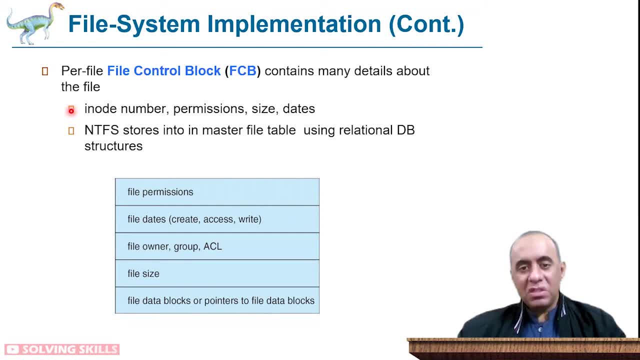 contains details about the file, like its id, their permission, size and dates. ntfs, by the way, stores into in the master file table using relational database structures. so the you can say and we will be looking at the fat structure in detail over here. but ntfs, the main difference, how the 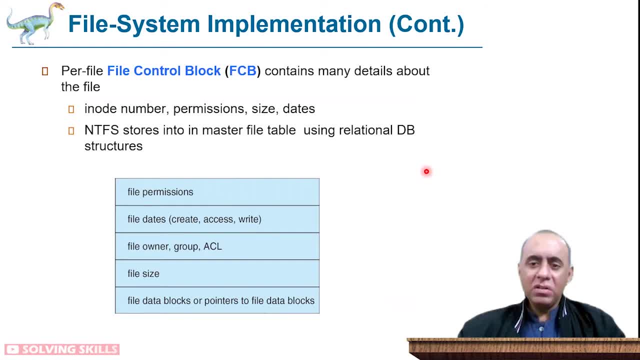 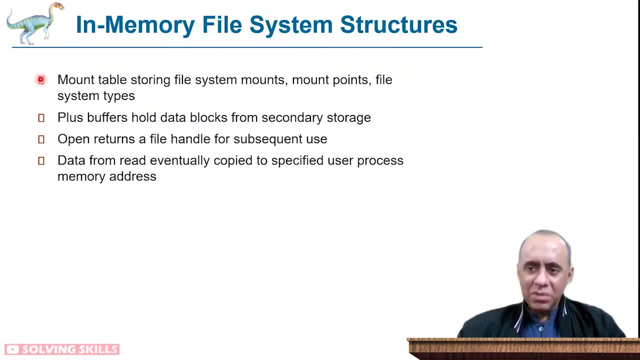 ntfs is faster than fat is that it uses advanced database structures to organize and maintain files. so whenever the operating system is running, everything that is happening inside the file is loaded into the memory. and once it is loaded into the memory, you can do certain things with those. 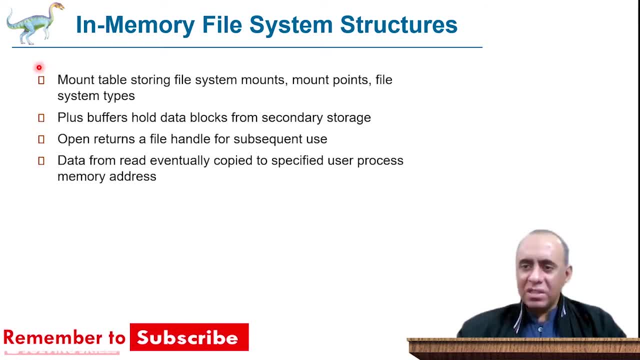 memory information about the file, so you can say the area that i shaded in the picture that i've been showing you you a lot of times, that a part of that is loaded inside the memory for fast access. so mountable storing file system mounts, mount points, file system types: these are loaded inside. 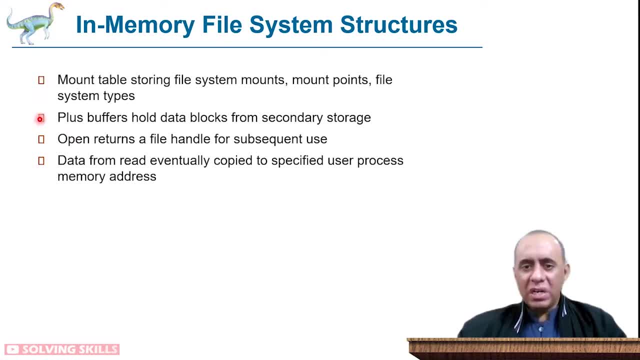 the memory buffers that hold data blocks from secondary storage. so obviously the an application program will be requesting a block from the operating system. so the operating system will be bringing that into its some kind of temporary memory, which is called a buffer, so that that the then it can be returned to the user that data. so openit turns a file handle for subsequent use. 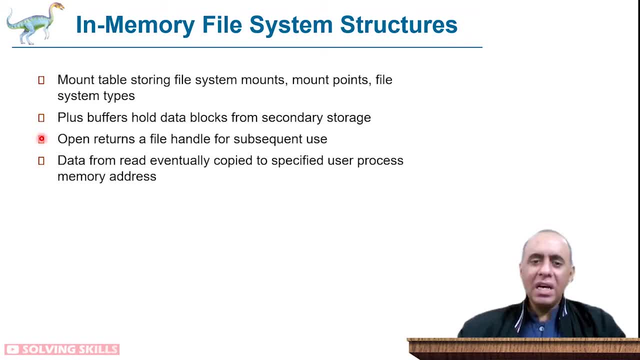 so this is also inside memory. whenever you open a file, a logical existence for that file is created, which is represented by the file handle and data from read eventually copied to specified user process memory address. so the the data which is transferred from the physical storage to buffers. 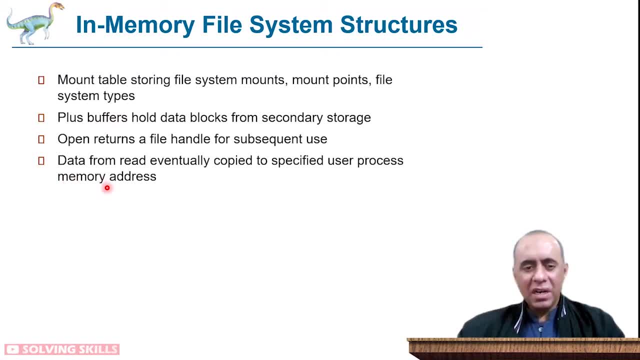 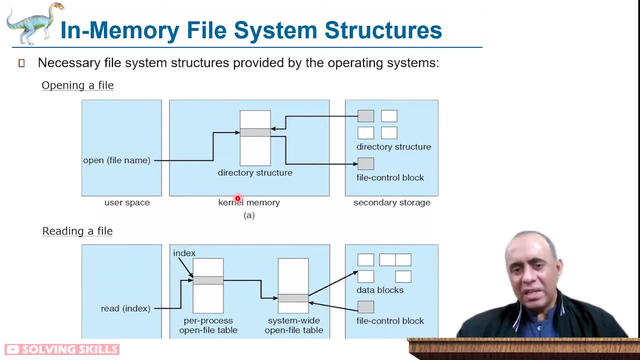 is then transferred to the user's address panel and the user's memory and the data is stored in the space the users processes address space. there are three things. this is the user space where the user is using system calls. then there is a kernel memory and then there is the physical. 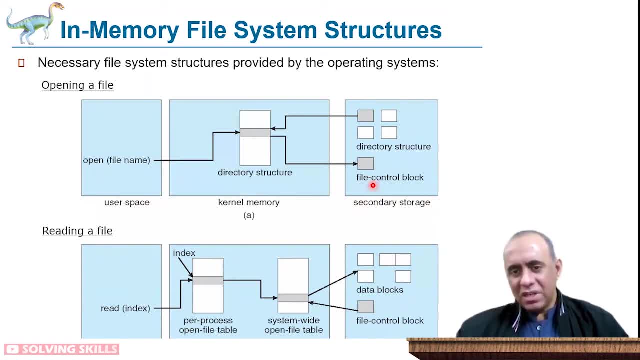 storage. inside the physical storage there is file system which contains the file control blocks and then there is the directory structure which manages how the files are stored and where the logical block numbers are stored. so the directory structure will actually be containing the logical block numbers, the physical location of all the file elements which are stored on the physical disk. 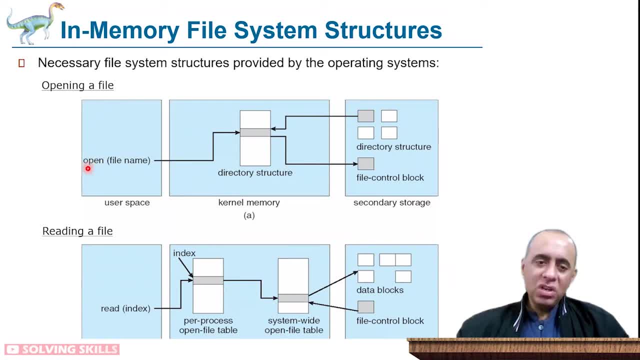 disk itself. so whenever the user uses the open system call, the directory structure is used to locate the file control block, and once the file control block is accessed, the kernel uses those the information, like the permission information and other stuff, to verify whether this user is allowed to use the current file or not, and then the directory structure is used to locate the. 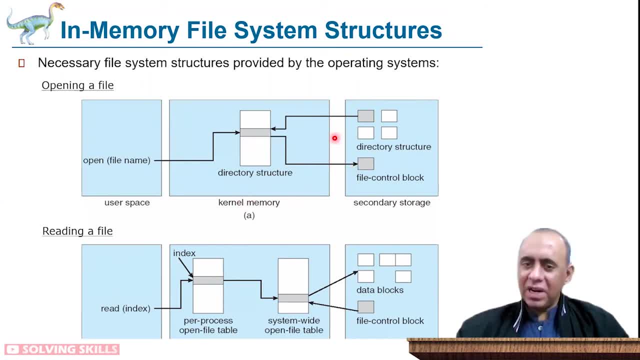 to you know, access this file and once the access is granted, the file control block tells which part of the directory structure contains the addresses for the logical blocks inside the disk. this file will be now entered into the opened files inside that kernel. but what? what do we do when we want to read from that file? so these are two different things, because 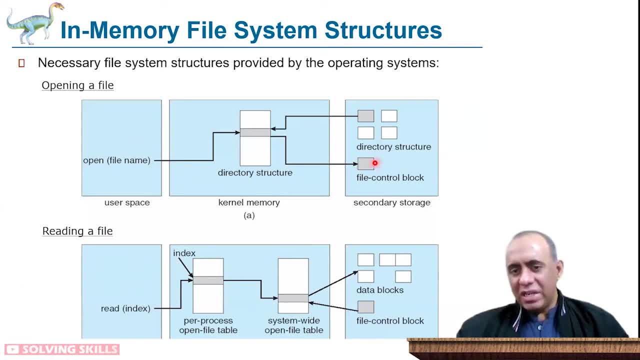 opening the file simply returns after validating the data. it simply returns the handle to the actual file inside the directory structure. but when you want to read to the file, read from the file, the read system call requests the operating system to read from that file and the operating systems looks for that file inside the open file table for that particular.